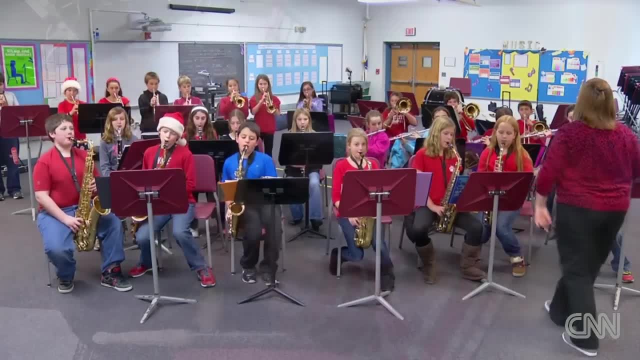 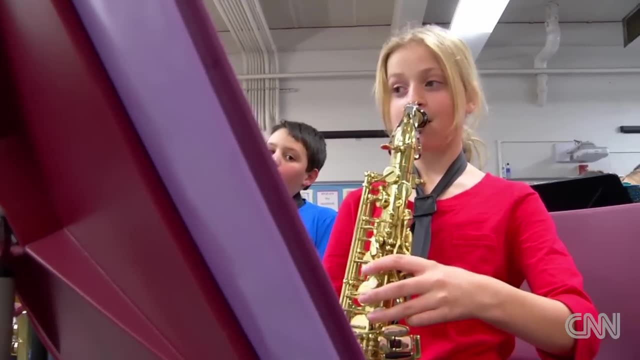 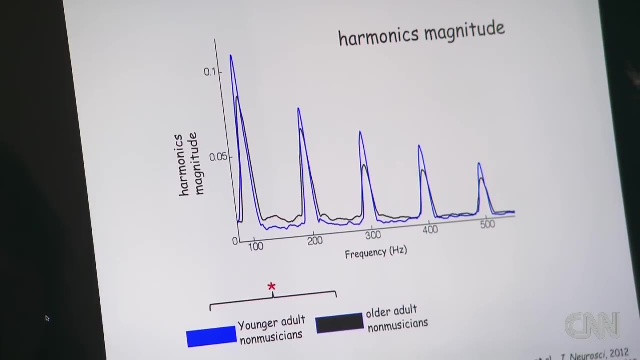 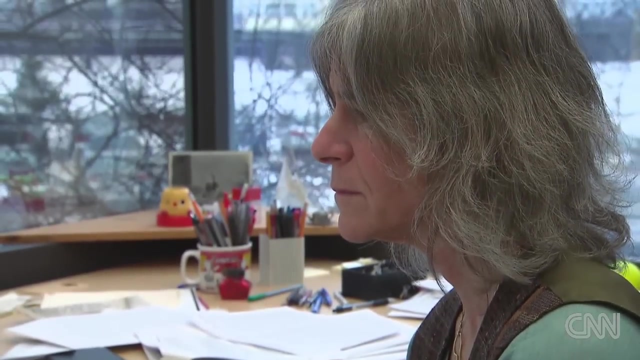 What's happening at the Miller Elementary School in Holliston, Massachusetts, may be more than what meets the ear. Researchers at Northwestern University have published several studies that show even limited childhood music lessons have numerous benefits for the brain. One of the most recent found older adults who'd studied music as kids had better neural timing and responded faster to sound later in life. 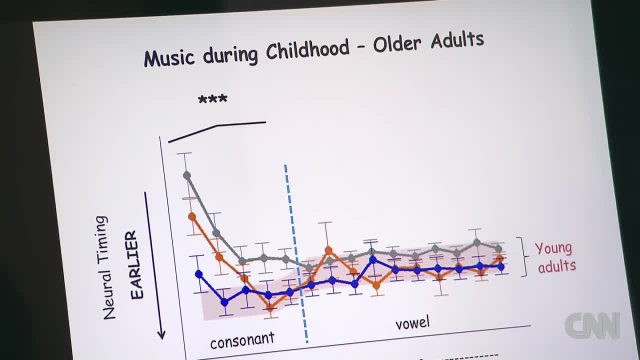 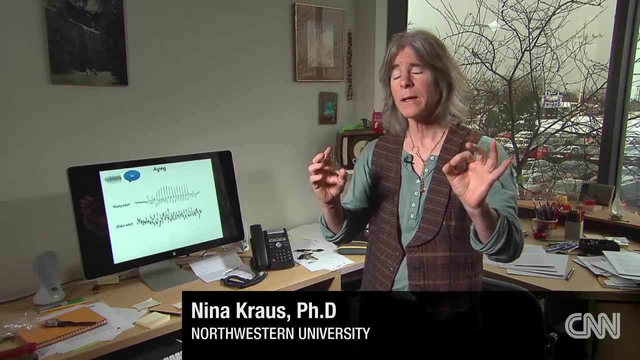 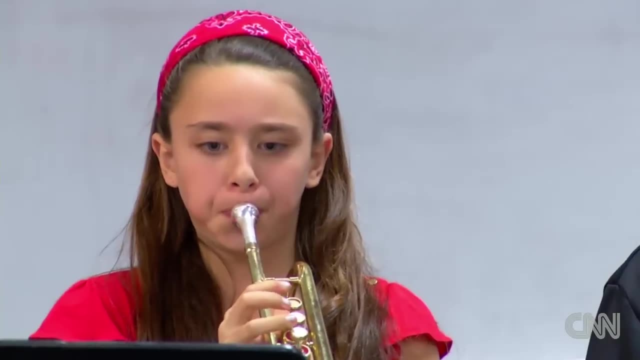 All key in keeping hearing and the brain sharp. These older adults with early musical experience have a biologically younger brain with respect to this particular responsiveness to sound, And the benefits of childhood music lessons seem to last Even if the person hadn't practiced for decades. 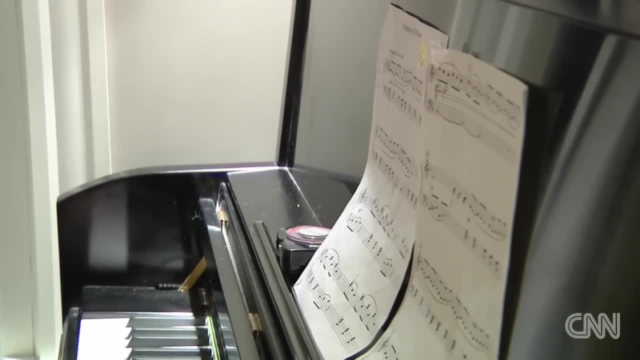 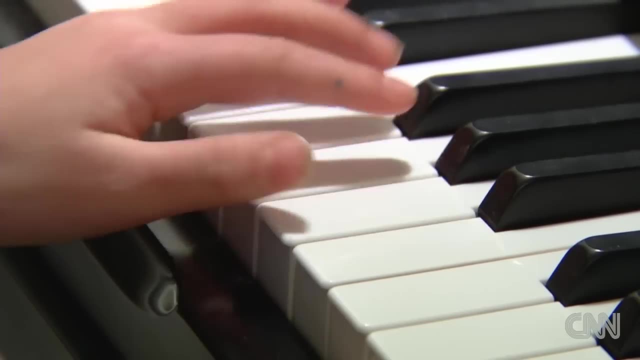 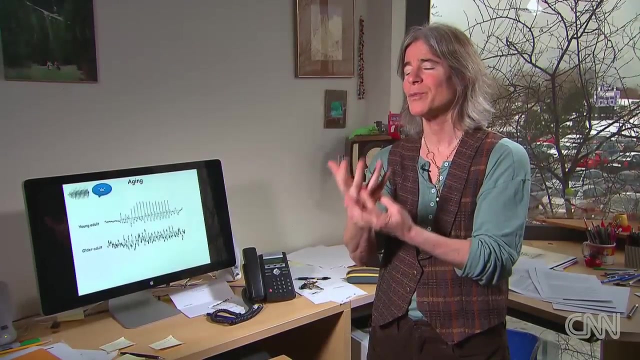 Other research from Northwestern shows children who study music become better readers and have better attention and memory skills. Kraus explains that just as exercise keeps the body fit, music lessons keep the auditory system fit. The auditory system is the temporal expert of the brain. 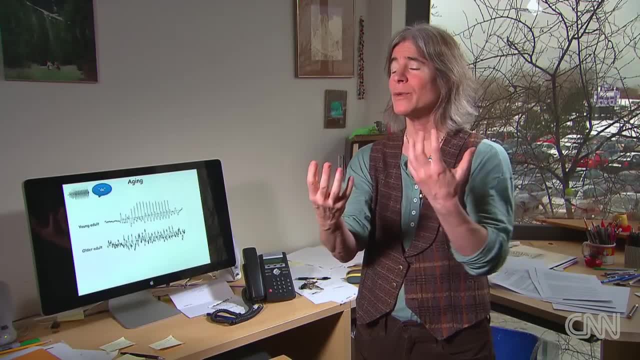 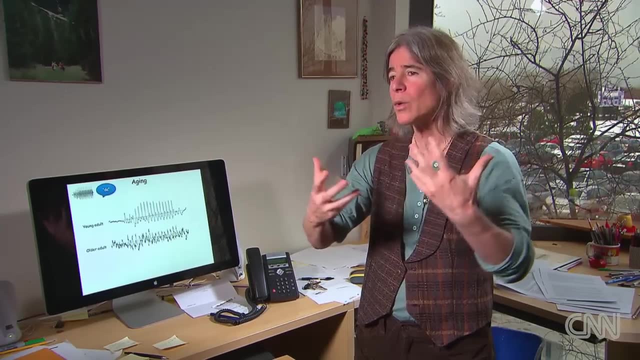 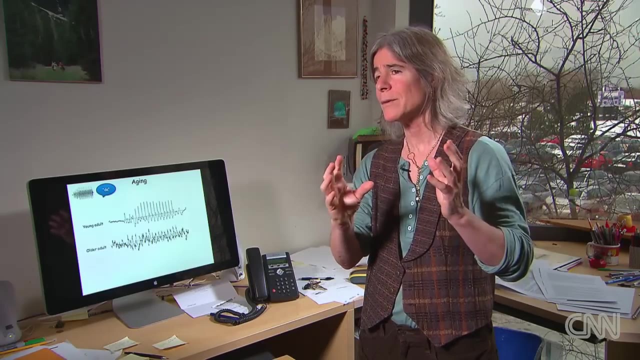 And we see that kids who have good reading skills, kids who have good hearing, kids who have good vision, kids who have good rhythmic skills and kids who play music are ones for whom sound is processed in a very consistent and stable manner. 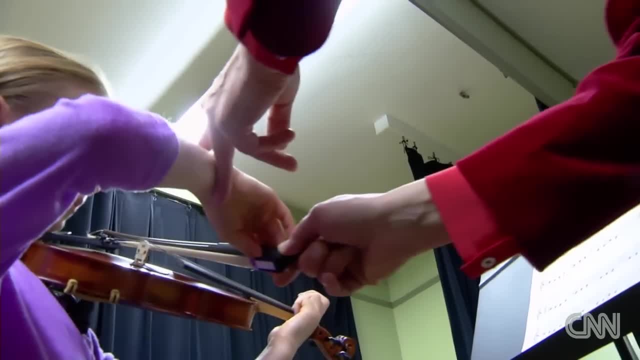 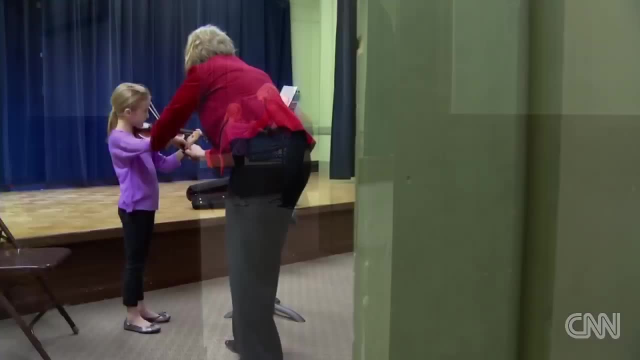 Irena Feinkeken is a musician and has been teaching children for almost 20 years. She believes all kids should be exposed to music because she's seen its powerful benefits firsthand. Ooh, what happened? And she has this advice for parents. 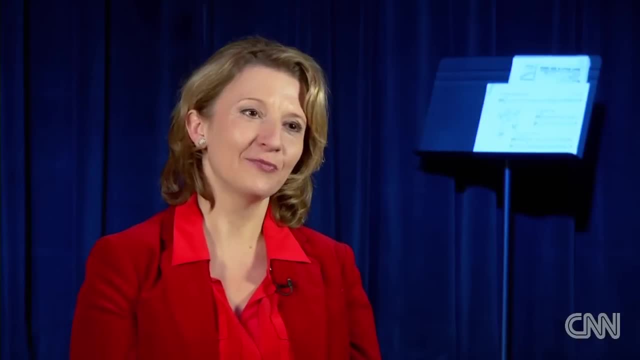 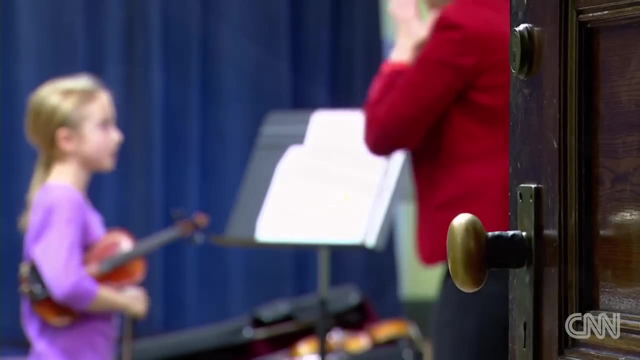 It seems to me that it's important not to quit And even if your child, for example, is not interested in playing this particular instrument, or you see that violin, for example, it's too hard maybe just to switch to a different instrument. 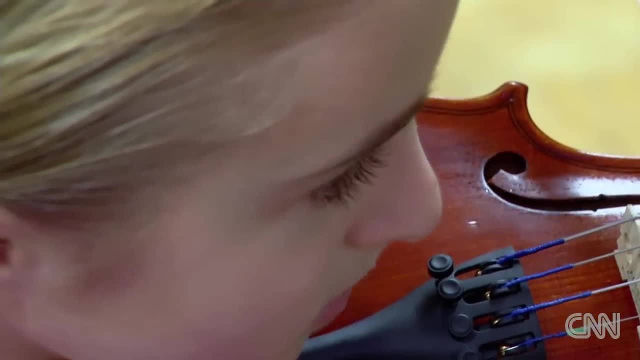 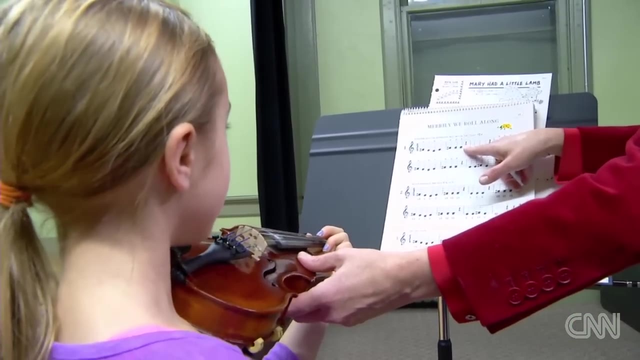 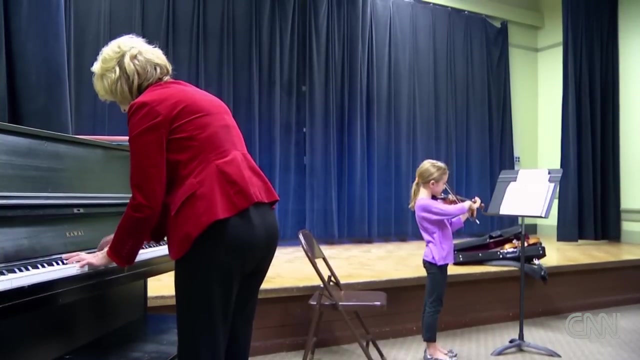 but still stay with the music because eventually it will give you a very good result. The good results don't come from simply listening to music but rather, say researchers, from learning to read and play, The actual engagement of playing the instrument of making, actively making those sound-to-meaning connections.